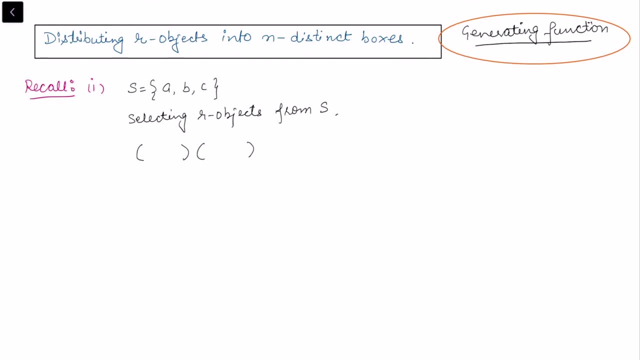 generating function. There are three objects. So I said that if there are three object, you create three parentheses and three product. This one is for object A, this one is for object B and this one is for object C. Now each object is appearing one. 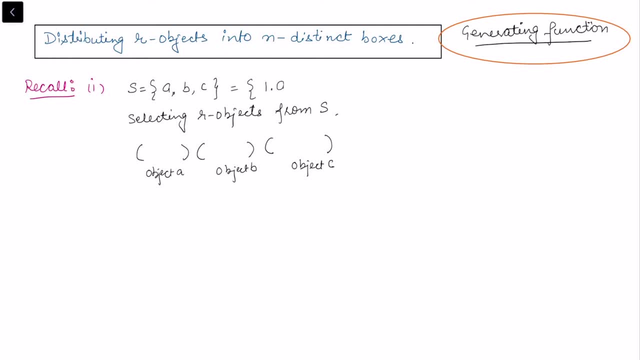 time In the multi set notation we could have written it as 1 into A, 1 into B and 1 into C, So each object is appearing at the most one time. So while counting we may consider 1 plus AX whole. 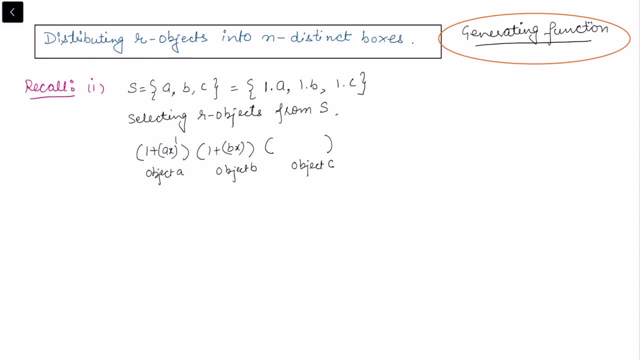 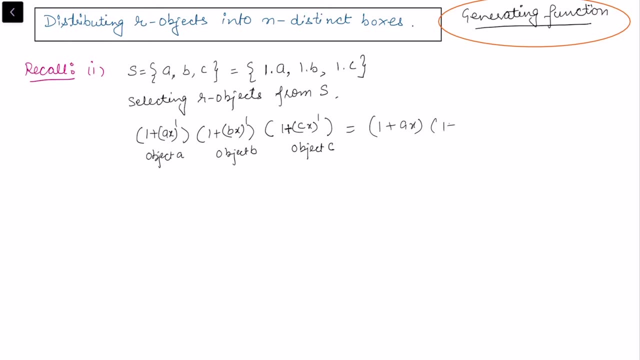 raised to power 1, 1 plus BX raised to power 1, 1 plus C X, whole raised to power 1.. Or we can say 1 plus AX into 1 plus BX, into 1 plus CX. This one means it is AX raised to power 0.. The object A is not selected. So this is how we have started. 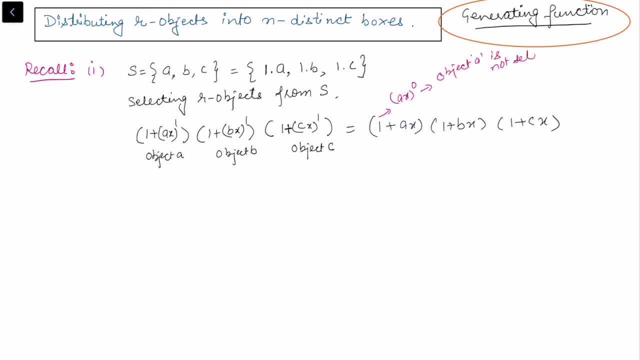 treating it. Object A is not selected And once you multiply this whole product we get in total 1 plus A plus B plus C times X, raised to power 1 plus. And then we take A, b plus bc plus ca x square plus abc x cube. this is means, if one object is selected, the exponent. 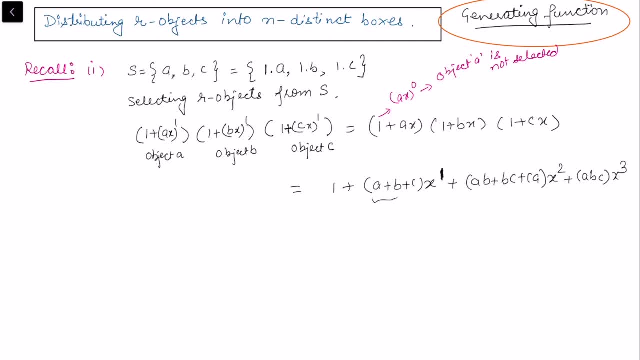 of x is per one means if the one object is selected. there are three ways and in those three ways i have here, when we read in this way, we are writing abc. so object: either object a selected, b selected, or the object c selected. the coefficient of x square gives me ab plus bc plus. 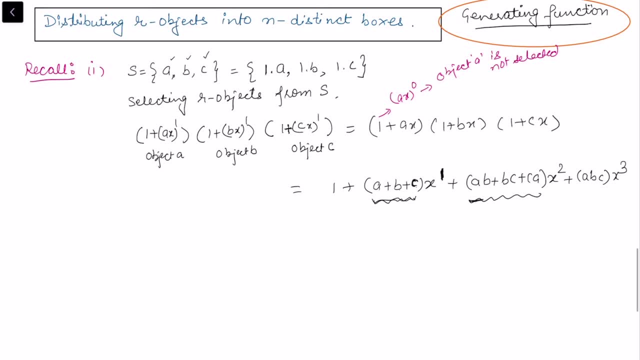 ca. so if two objects are selected, either ab selected or bc selected or ca selected, and so there are three ways. so in case we simply want to know the counting of the selection, or we want to see how many ways we can select, okay, so number of ways of selection: in this case we simply have. 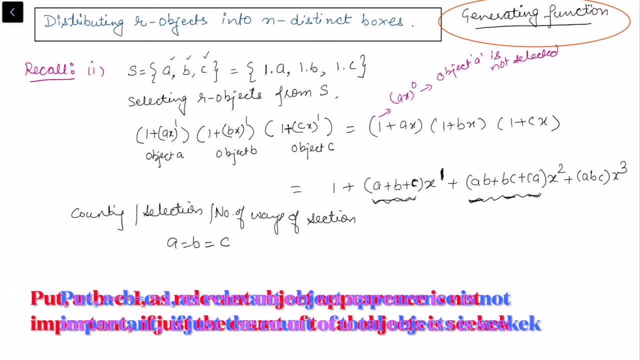 written a equal to b, equal to c, so the generating function reduces to one plus. if you substitute a plus b plus c equal, so you get three times x to the power, one plus three times x square plus one times x cube, and this is essentially the same as if we write the out of three object we 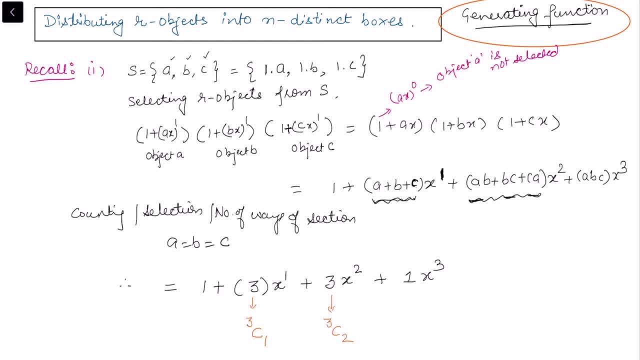 have selected one out of three object. we selected two out of three object. we selected all three at a time, and for this we know there are three ways. for this there are three ways and for this there is one way. so this way we can look at the generating function. now i'll be recalling one. 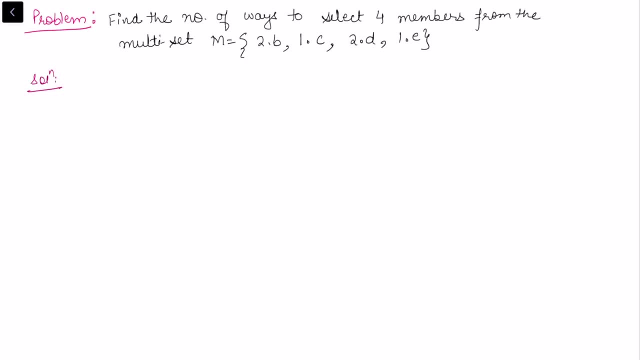 more example before coming to the distribution problems, and here find the number of ways to select four members from the multi-set. this, and in this case we can see how many objects are given. so there are four objects in total given to us, and then, of course, each object like the first. 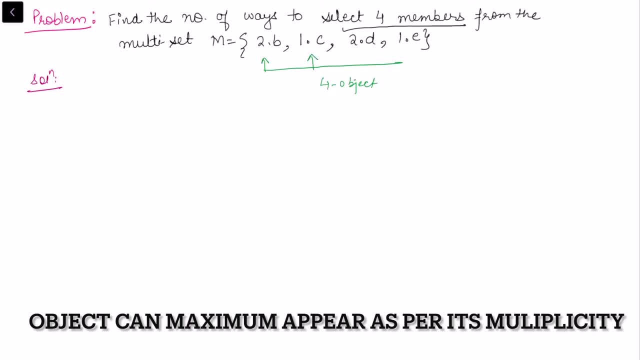 object is appearing two times, this c can appear one time and d can appear two times and e can appear one time. or it is like b can repeat two times, c can repeat one time and d can repeat two time and e can repeat one time. so in the multi-set notations we always write the project into distinct format and multiplicity. 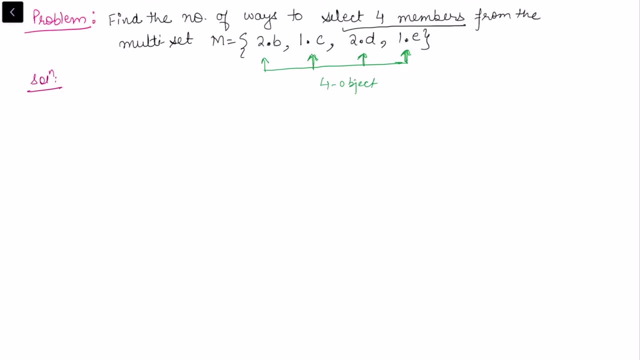 comes in here with the objects. so for this, the generating function, we can write as per the above, there are four objects, so we will have four, parent this is. and then, based on four, we have to see first object. two copies can come, so if no copy comes, it is one one. into x: raised power zero. 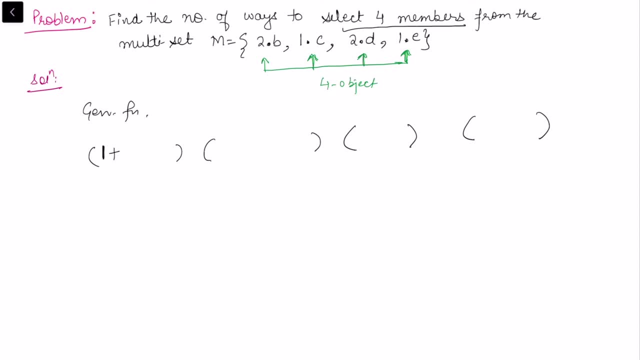 and also now i'm not interested in knowing the relevant case. so, corresponding to each object, b, c, d, e, we are considering, so we, i'm already considering b equal to c, equal to d, equal to a. so the object value is one, we just we need to know in how many. 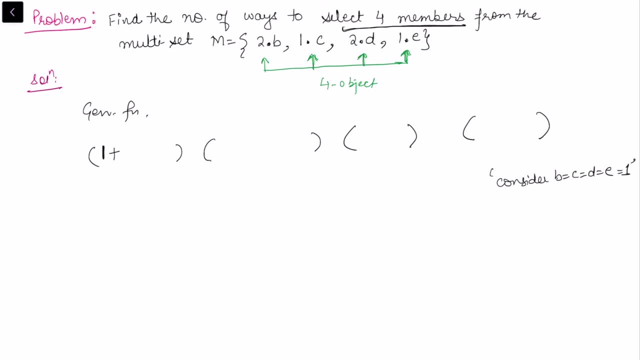 ways they are going to give me four selected members. so we'll have one plus x plus x square. this is corresponding to object b, then corresponding to object c- you can see that one. it can appear one time. so we'll have one plus x to the power one. this one means it is not coming and this x to the power one means it is. 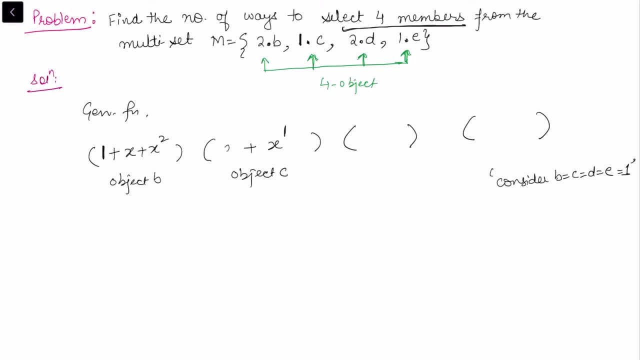 appearing one time. we can also write this one as x to the power zero, so zero times it is a pairing. or we can simply write it as one, then object d, so we can see again, it is two times. so one plus x plus x square, and object e: one plus x. so that's the generating function. now, multiplying this generating: 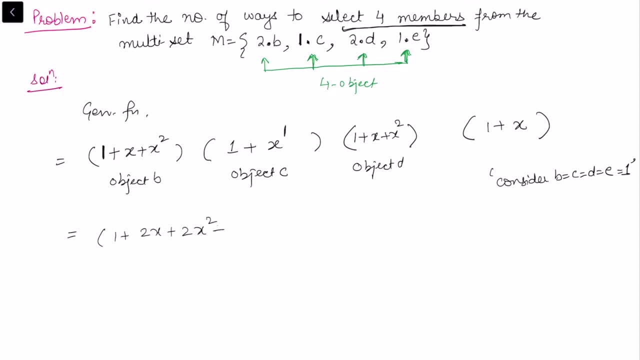 function, we get one plus two, x plus two, x, square plus cube and the remaining terms. when i multiply, we get this term. now we are interested in knowing the coefficient of x to the power four because we are interested in how many ways we can select four. four can come due to different combinations, so four can come when this x is multiplied by this. 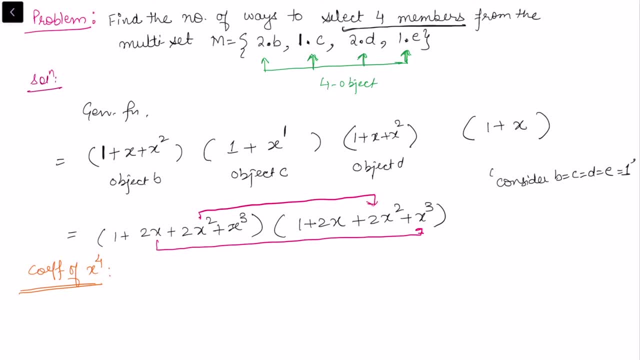 x cube. this x square is multiplied by this x square, or this x cube is multiplied by this x. so, looking at these, we see a4. this is equal to two plus four plus two. that is eight. so a4 is eight. so we can say there are eight ways. 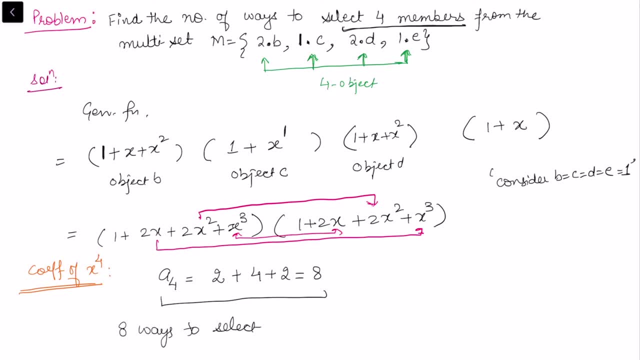 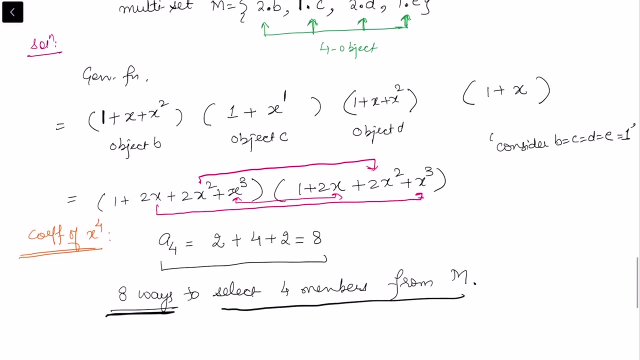 to select four members, four members from the set m. so this eight way is simply the counting, the number counts to select four. object: and if you are also interested in knowing what are the relevant eight cases, if somebody was interested in the relevant cases, in that case you could have considered the generating function. so consider: 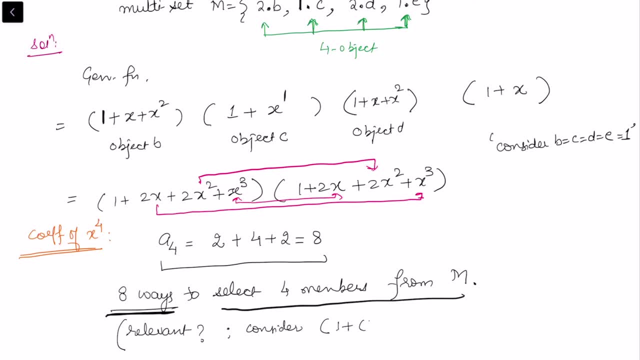 the generating function in this order: one plus b x appearing one time plus b x appearing twice. this is for the first object, then this one is for the second object, this one is for the dx and then dx square. this one is for the third object. multiplied by one plus e x raised to power. 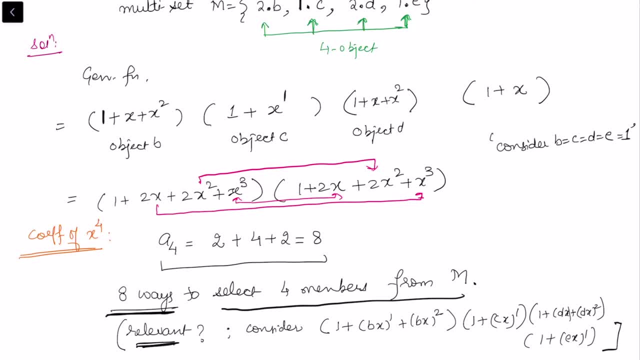 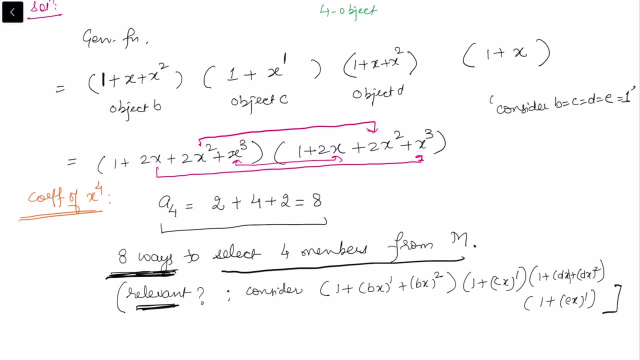 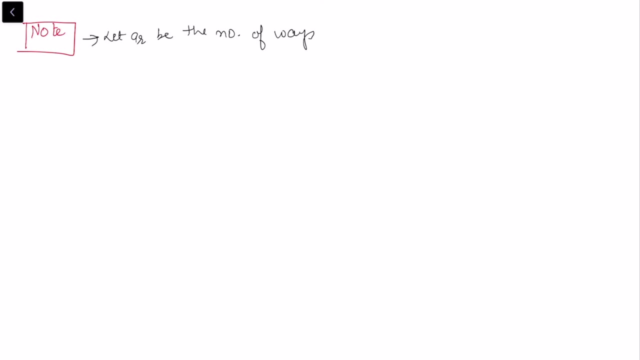 one. this one is for the last project. if you want to know the relevant cases now, if you take the product, we will see that there will be eight possible ways that we can trace it from here, just like i have explained in my last example. so we can note that, in general, if we want to consider that at ar, this be the 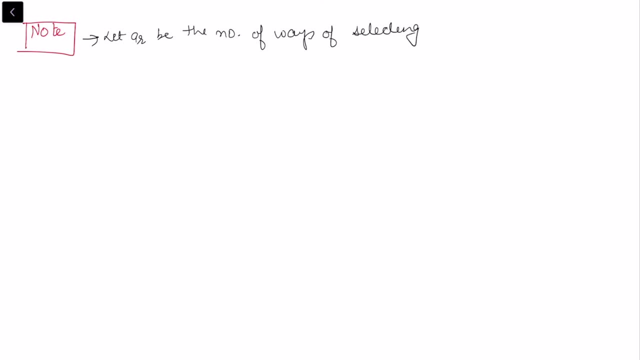 number of ways of selecting r members. r members from the multi set m, which is equal to, in which the first is coming n one times, second is coming n two times and the kth object is coming n k times, then generating function for the sequence ar. this is given. by now you can see that there are k object given in the set. so 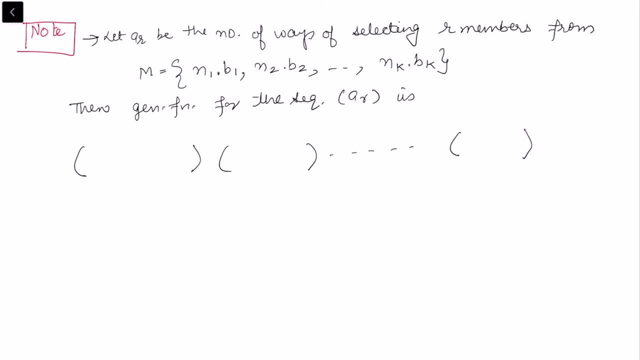 just create k products and the first product one plus x, plus up till so on, it will go maximum till n one, because that's the objects. repetition available in the set b one is repeating maximum n one times. and similarly for the next case, plus x, raised to power n two, and for the last case, x. 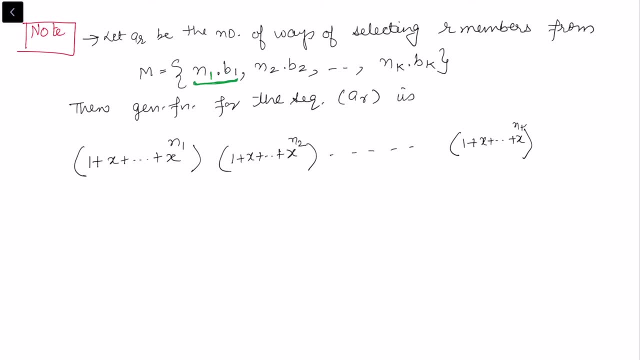 plus, so on, so on, so on, plus x, raised to power n, k, and so here we can read them: so ar, which will be actually the coefficient of x to the power r, this will depict the number of ways of selecting r object, of selecting r members or r elements from the set m. and in general, if we 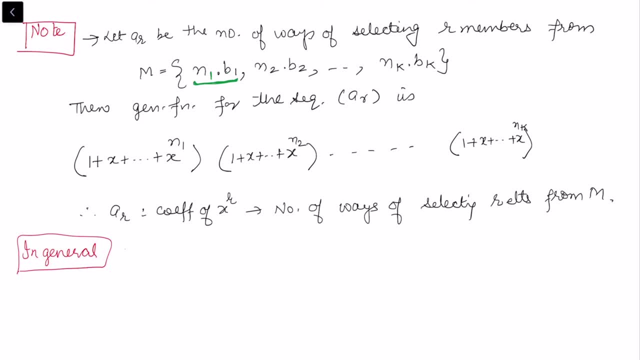 extend. suppose the supply is infinite in general. suppose the set that we have considered, let m. this is infinity. so infinity is just a notation here. infinity comma, b one. this means b one can repeat any number of time, infinity into b two and so on, up till infinity into b k, the only change in this. 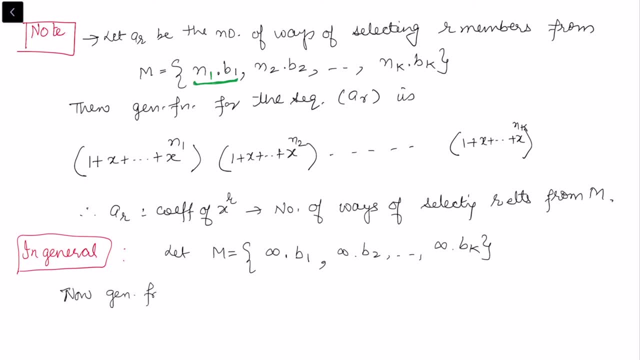 now the generating function become so: one plus x plus, so on, up till so on. there is no restriction here, because we know that this supply is infinite. and then for the second object, we will continue, for the third object, we will continue, and so on. for the last, that's the kth object, we will continue. 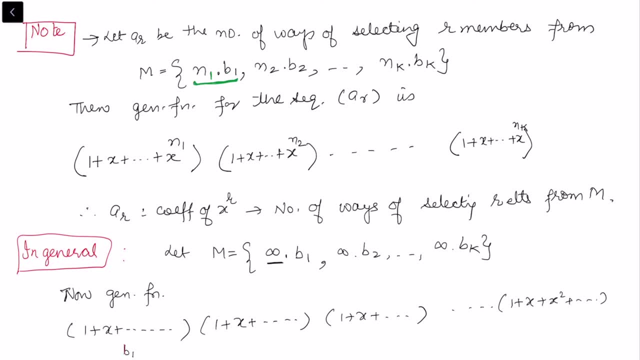 so this one is for b one. we can write down: this one is for b one, this one is for b two and this one is for b three. and we continue to write down: this one is for b two and this one is for b three. continue. this one is for bk. now for the infinite series. it is more easy because we have a more nice. 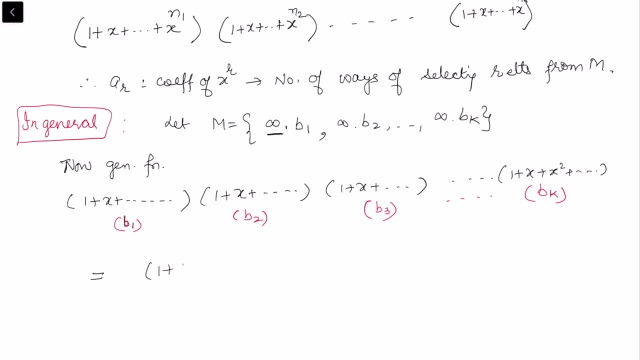 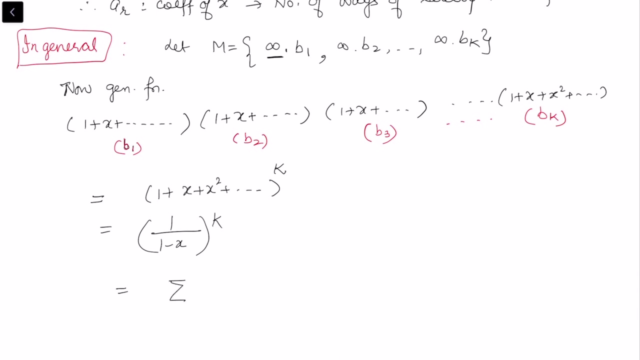 closed form structure. we can see that this become 1 plus x plus x, square plus on up till raised to power k. so there are k terms and then so this is same as 1 over 1 minus x raised to power k using the gp formula and now using the binomial expression, i can write this as summation: r goes. 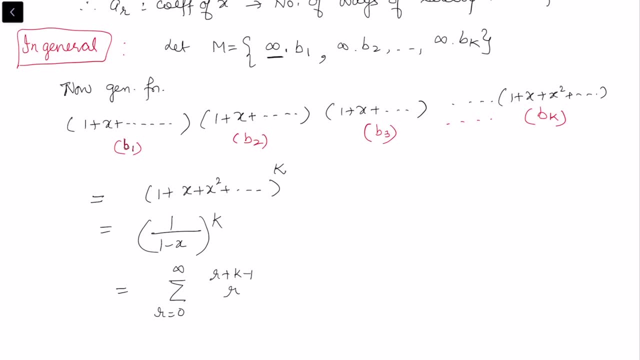 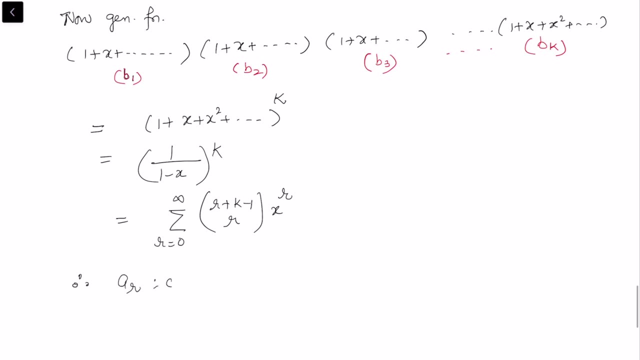 from 0 to infinity. r plus k minus 1. choose r. x to the power r. so from here i can trace. so ar, this is the coefficient of x to the power r, and that is same as r plus k minus 1. choose r. so in the if the structure is infinite, here infinity is the supply. each object is appearing. 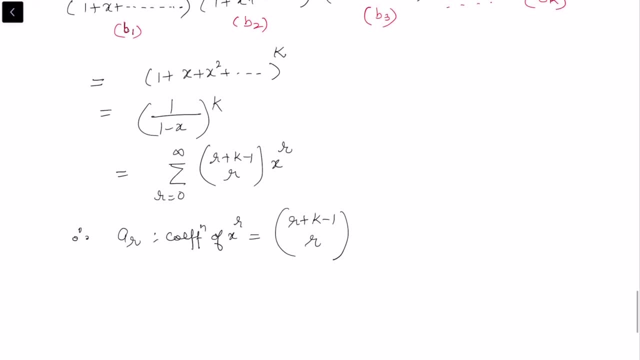 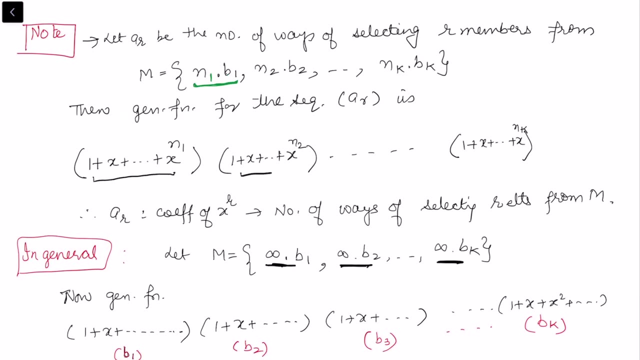 as many as number of time, we can find a very nice formula for ar, whereas in case of the finite- so suppose. if this was so- we need to apply the finite gp formula for each of the term, and then we need to understand the coefficient corresponding to individual and we need to 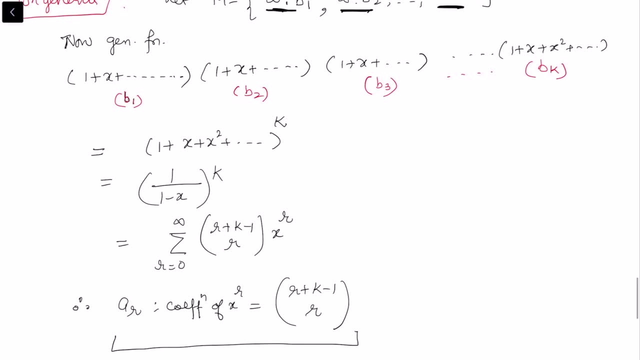 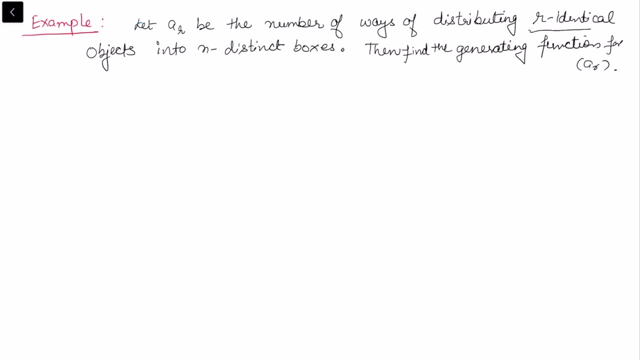 multiply, but of course for the infinite this closed forms becomes more, nicer and more easier to understand. now, in this example, let ar be the number of ways of distributing r identical objects into n distinct boxes. so if we just compare it from the previous example, in that case we have 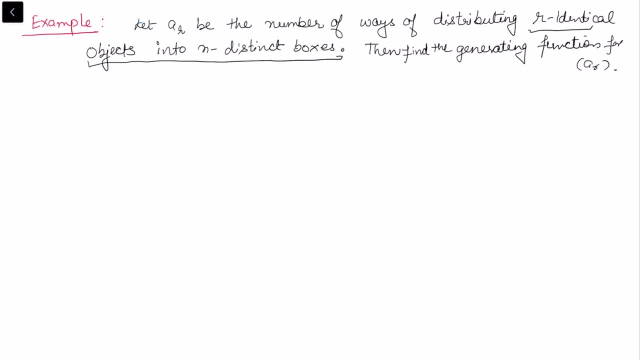 used the parenthesis. this is like, for example, in the set m we said that there are k objects, b 1, b up till bk, and so we created k times of the bracket. so these parenthesis, we created k times, and each depends upon the multiplicity of the each object. so here, 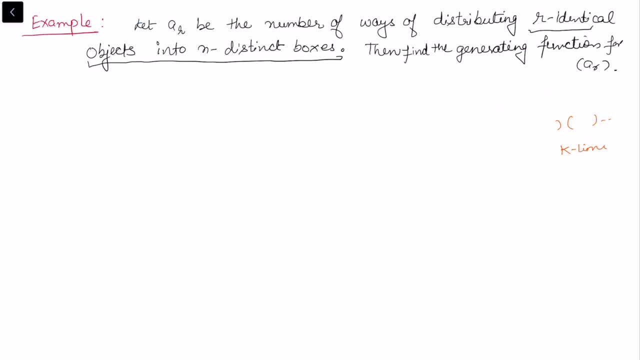 what is the difference is we have n distinct boxes. so that means in the multi set the quantity that we are considering is has to be distinct available. so I'll start considering from n distinct boxes. so in this case the generating function can be written it as: consider it as box 1. so this is for. 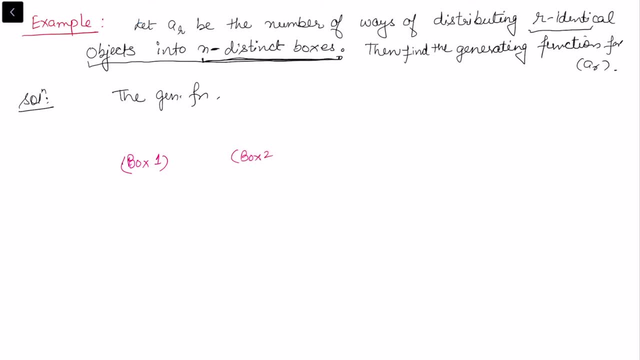 box 1, and then we consider it for box 2 up till so on box n. so we have already considered the distinct part here. now we want to place here the objects which are coming in these boxes, and we have to also see the multiplicity in these boxes. now you notice that we are saying that ar be the 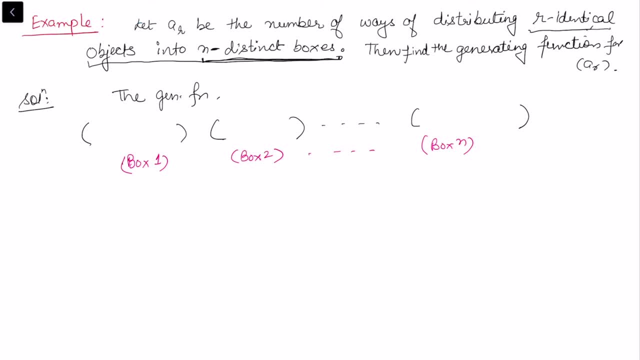 number of ways of distributing r identical objects into n distinct boxes. so it is possible that in the first box that identical object is not appearing. so that means the value is 1 or x raised to power 0, or the object is appearing one time, or the object is. 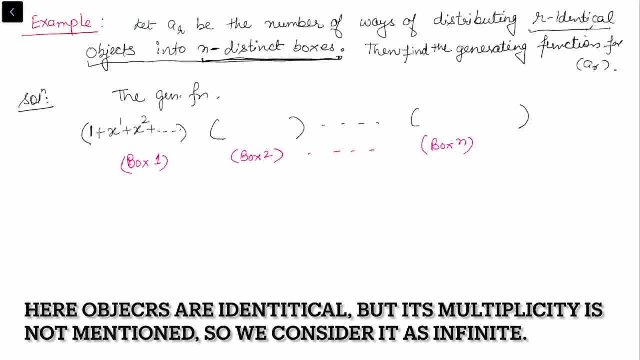 appearing two time, and so on. so the supply is infinite. similarly in box 2 the object may not appear, it appear once, it appear twice, and so on. and here also the object is appearing once, twice, and so on. so what we get? we get 1 over 1 minus x, whole raised to power n. so this problem is same. 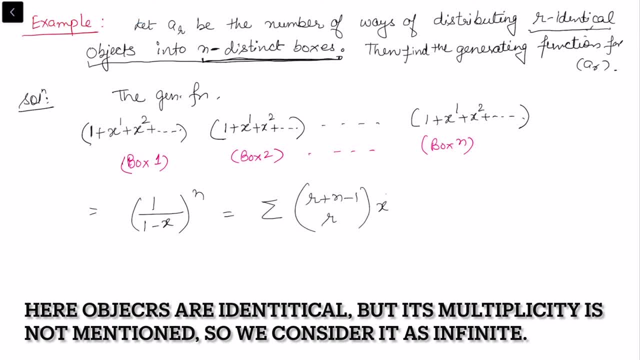 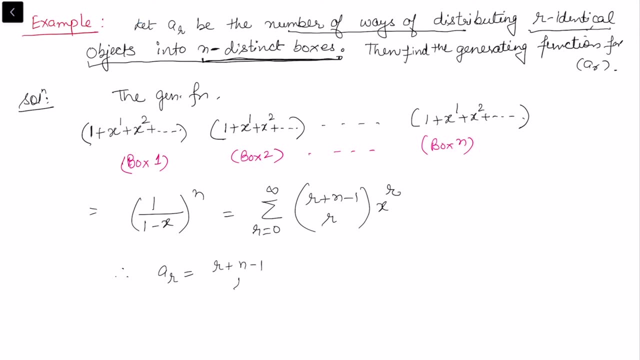 and introduces to the same problem, so the one that we have just discussed earlier. so this become r, goes from 0 to infinity, and so we notice ar, that is, the number of ways of distributing r identical object into n distinct boxes, is same as r plus n minus 1. choose r. now consider this example, and in this we have only an addition in. 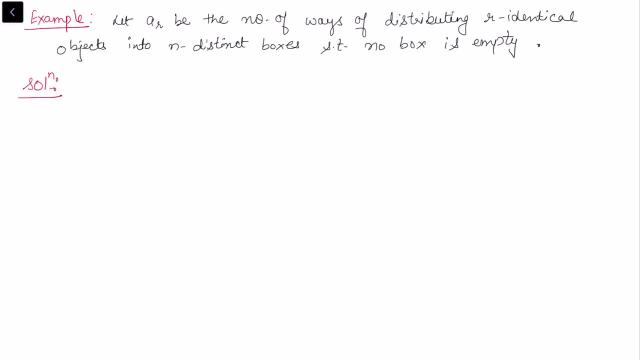 the problem that we just discussed let ar be the number of ways of distributing r identical objects into n distinct boxes, such that no boxes are going to be able to be distributed into n distinct boxes. so first we need to count that the box 1 and n distinct boxes are存 in n this thing that is. 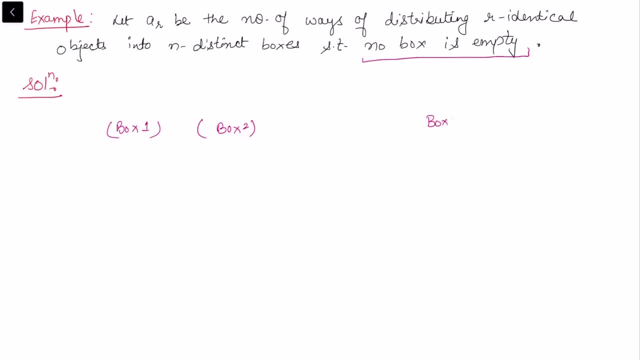 empty. so for that, we have just seen that there are n distinct boxes. so let's first place the distinct things, box 1 up till box n. now in these boxes we said that if an object, an object may appear and an object may not appear. if it is not appearing we will say that one is coming, so x. 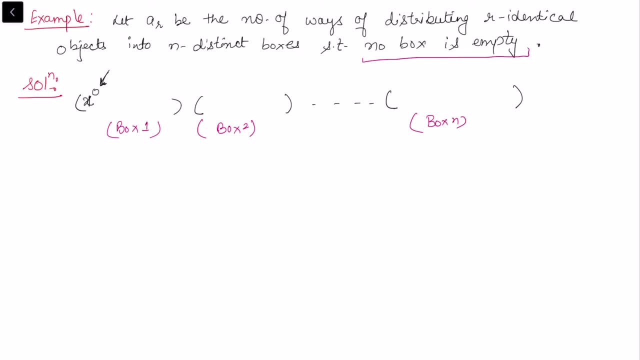 raised to power zero. this 0 means the object, object appearance is nil. so this is the and anything throat to. the power 0 variable will correspond to the constant term, that is 1 plus x, to the power 1 plus x square. that was a normal way of conducting, but here we said: no box is empty, this means every. 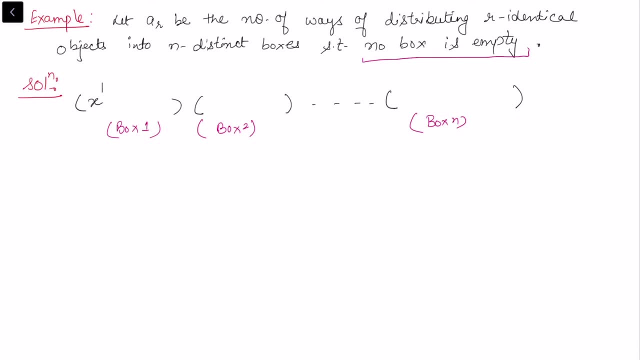 box has at least one object. so we will start it from x to the power 1, not from the constant term, that is, x to the power 0. so x to the power 1, x square. and then we can supply as many as number of time. similarly in box 2, box 2 cannot be empty. similarly the box n cannot be empty. so in total, 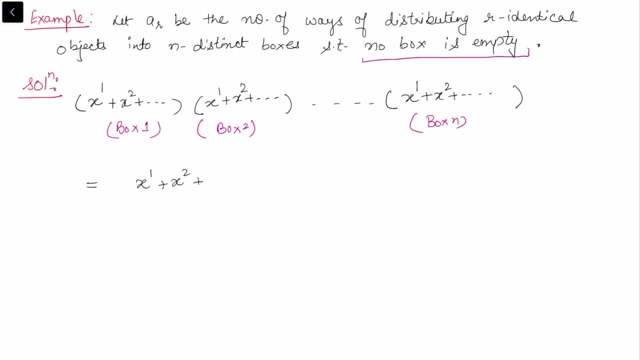 we will have x to the power 1 plus x square plus, so on, raised to power n, and now we can see that we can take x to the power 1 common from everywhere. so outside, let me do okay, let me write here this one as x into 1 plus x plus x square plus, so on. 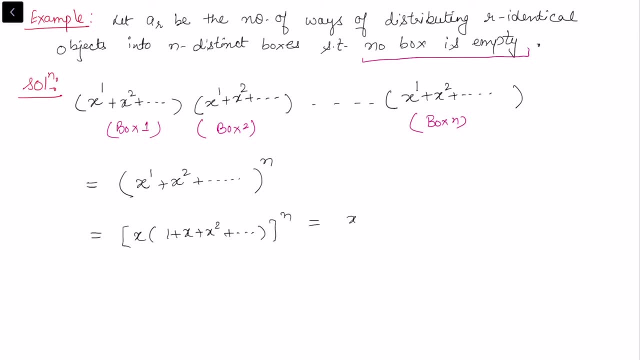 okay, whole raised to power n, and then we notice that x to the power n comes outside and inside we have a 1 over 1 minus x raised to power n, and this is same as x to the power n. this is summation i varying from 0 to infinity: i plus n, minus 1. choose i x to the power i. now i have explained in one of 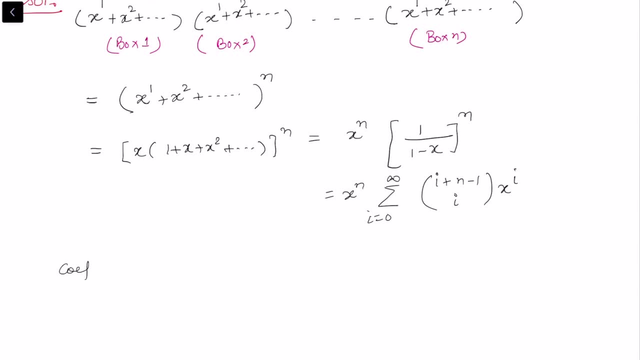 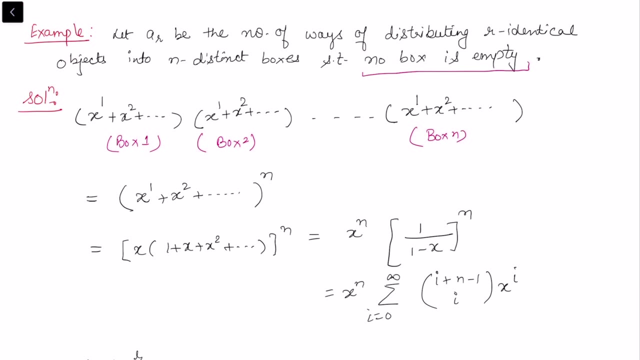 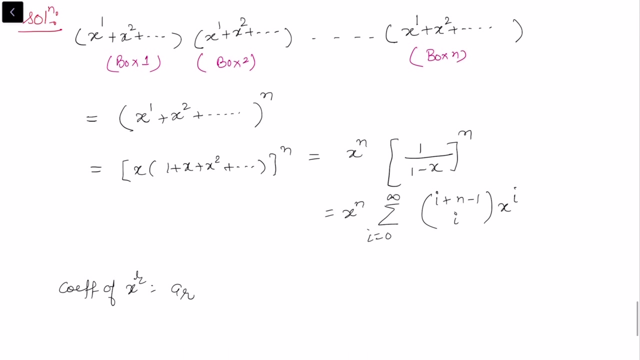 my previous videos that if you want to find the coefficient of x to the power r, that is ar, because this will give me the. ar is the number of ways of distributing r objects into n distinct boxes, with this condition that no box is empty. so we are interested in knowing what is the coefficient of x to the power r? what? 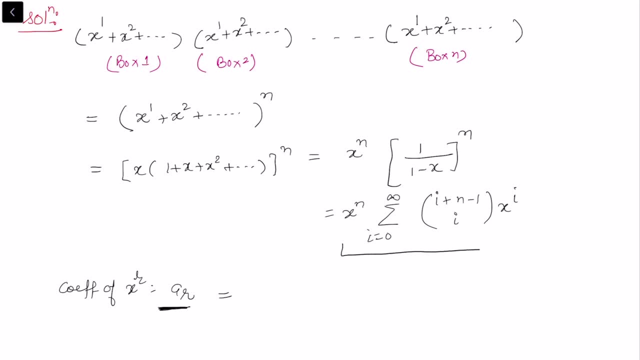 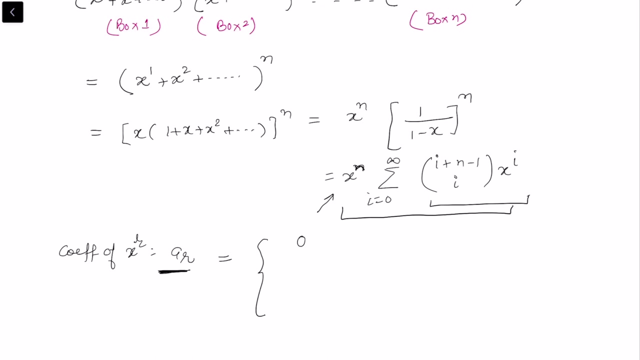 is ar. so i want to look the coefficient of ar in this case, and we notice that x to the power n is already multiplied. so we want to see inside n some coefficient subtracting this value. and then we want to see what is the r. so ar, this is zero if r is 0. and if r is 0 then we want to see if r is 0. 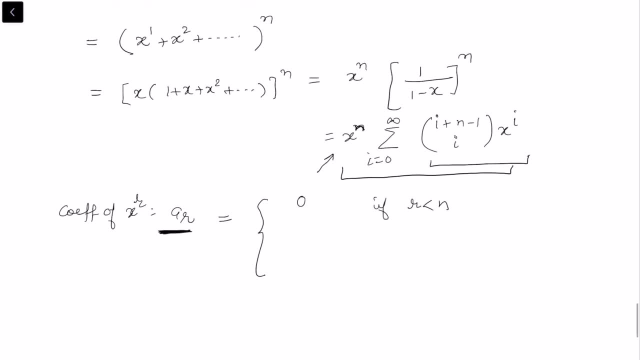 is less than n. so if it is less than n, I'll take a particular case to explain this part. so this is r minus 1 plus n minus 1. choose n minus 1, which is same as r minus 1. choose n minus 1 if r is. 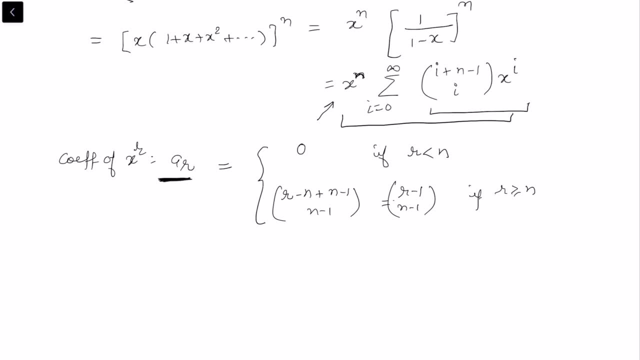 greater than equal to n. Now to see this case, what do I mean? say n is equal to 3, this means x cube here in the star. for example, in star x n is equal to 3. and then you're looking some coefficient i varying from 0 to infinity. i plus n, minus 1. choose i x to the power i. so when you open the series, 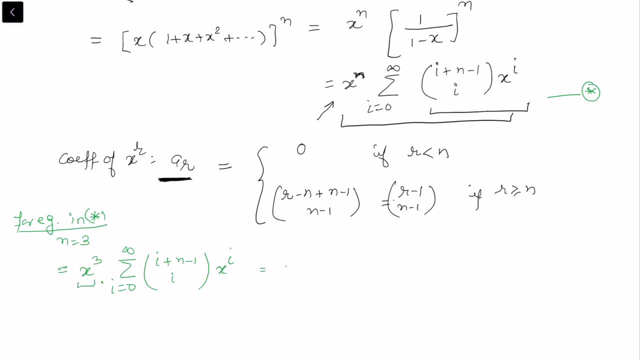 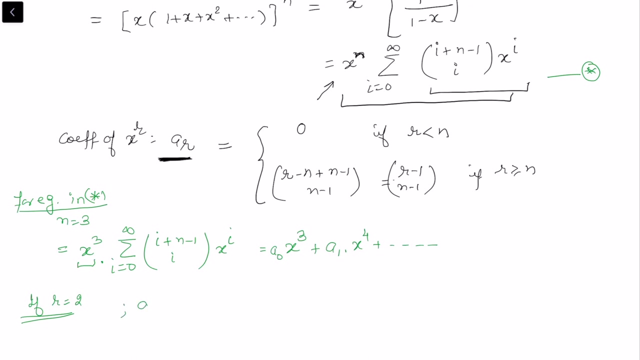 this means every coefficient start. this means the series actually start from x cube, so there will be some coefficient, a naught, then you'll have a1 into x to the power 4 and so on. so if we are searching, if r is equal to 2, then of course a2 is a 0 because there is no coefficient of okay. so in 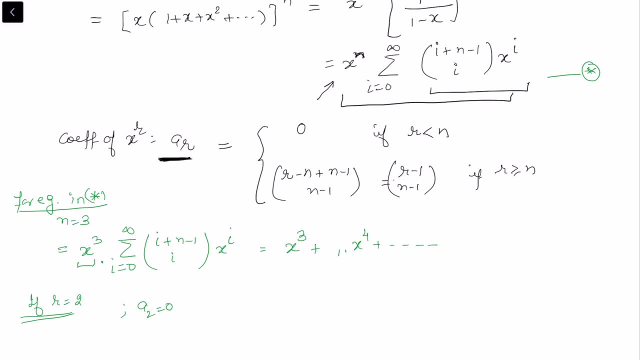 this case we may consider this one as b naught b1. let's say, if this coefficient is considered as b naught b1. and now, if r is equal to 2, we can see that there is no coefficient of x square in this series, because the series start from x cube. so a2 is 0. this is what is written here. if r is less, 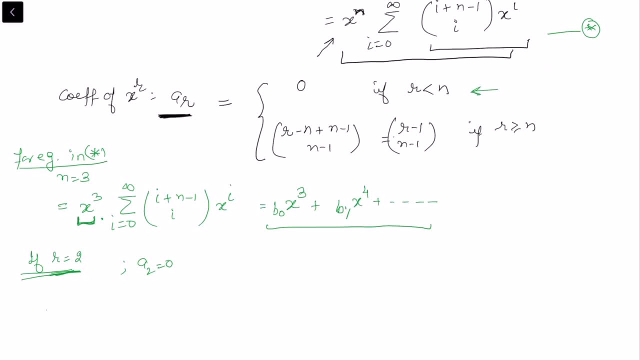 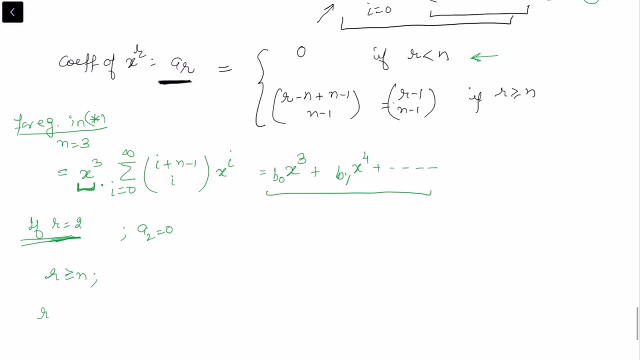 than n, a r is 0. so whenever r is equal to n or it is strictly greater than in this case, now suppose i want to take, r is equal to 5. so if r is equal to 5 and we notice that x cube is here, and then we have some term, i plus n, minus 1, choose i. 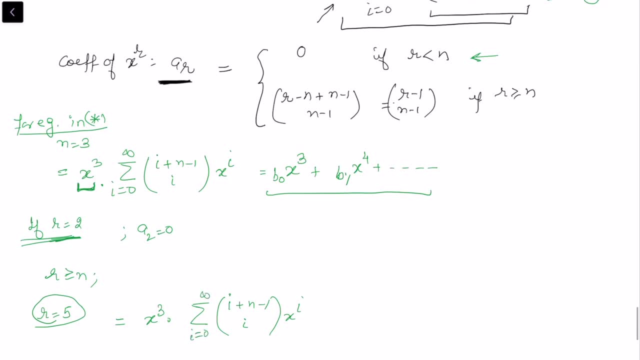 x raised to power i, i varying from 0 to infinity, x cube is already here. this means i i'm only interested in knowing the coefficient of x square from here, so that x cube multiplied by x square total, i am getting a coefficient of x2 to the power 5. this point i have already explained: how to find the coefficient or how to look for. 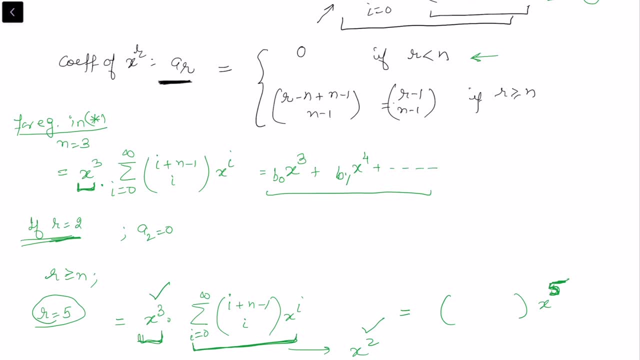 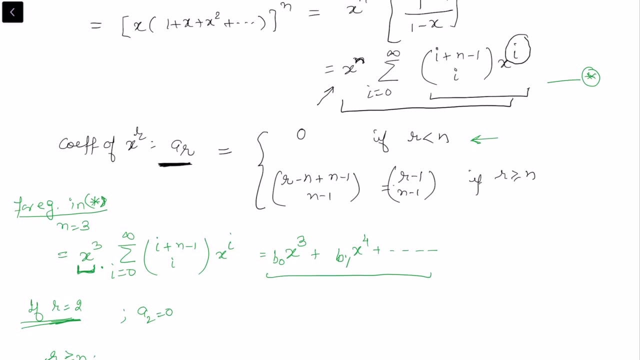 the coefficient in an expansion link added in description. you can please see the previous video first. so now, instead of this, i, since i'm looking for the coefficient of x to the power r, what i will say is: look for r minus n, because then when you add this plus n, this actually becomes a. 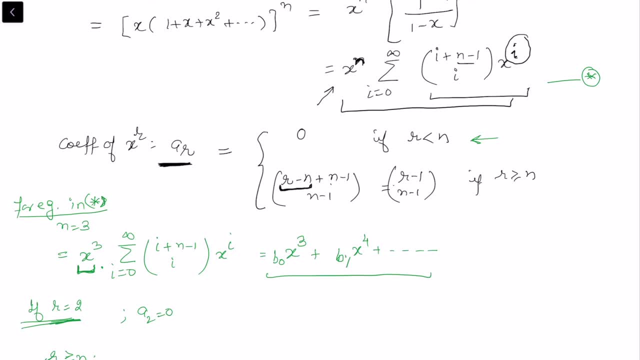 coefficient of r. so the remaining terms is same. this is n minus 1, And here also you can write it as n minus 1 or r minus 1, because i plus n minus 1, choose i. This is same as i plus n minus 1, choose n minus 1.. 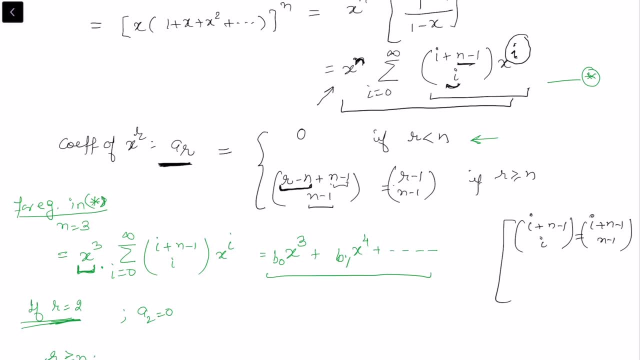 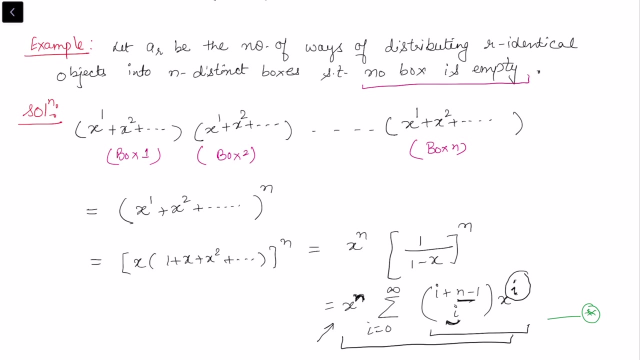 So this is same as n minus 1, and when you simplify we get r minus 1. choose n minus 1.. So by looking at this we get the nice formulas for handling these problems where we want to distribute our identical objects into n distinct boxes, with no box empty, and here is the generating function corresponding to this one. 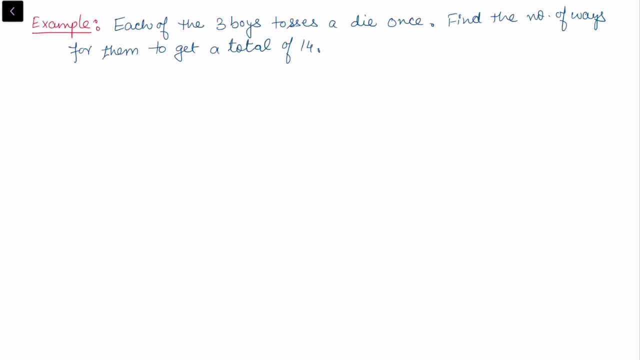 So we consider one more example, and in this each of the three boys toss a die once, and we want to find the number of ways for them to get a total of 14.. So again, I am doing this problem using the generating function. 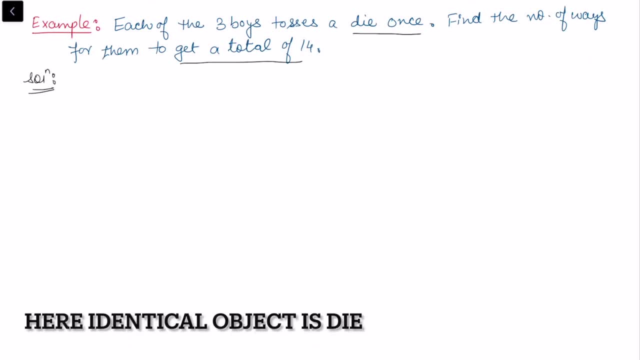 So while writing the generating function, we must need to look at which is the things which are considered distinct, So that by looking from the previous expression we should create parenthesis for the distinct object and then we should generate these quantities. So now here, three boys are considered as distinct. 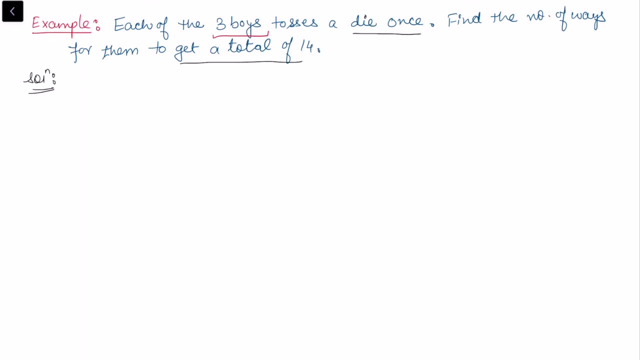 Obviously, people are considered as distinct and they are tossing a dice once. So we will write the generating function and we want to know what is the total of 14.. So let's see. So let A R, this be the number of ways to get a total of R, and later on we will take the case when R is equal to 14.. 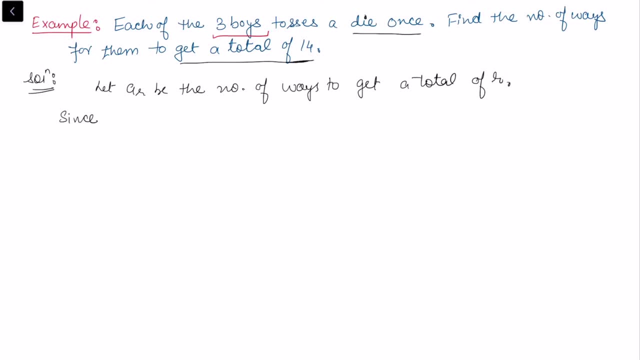 And we also know that the outcomes for the dice are, since outcomes of tossing a die are: either it is 1,, 2, 3.. 4,, 5, or 6.. So these are the only possibility. So for this we have the generating function as 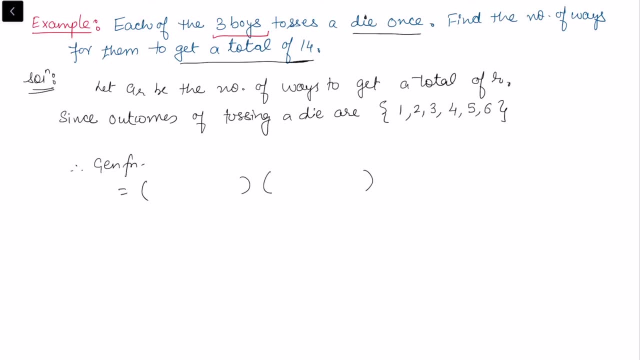 Now, this is of course for the three boys. So I am creating for the three boys. It is possible that the first boy get on the dice as 1.. Second boy- sorry, the first boy get on the die as quantity 2 and 3.. 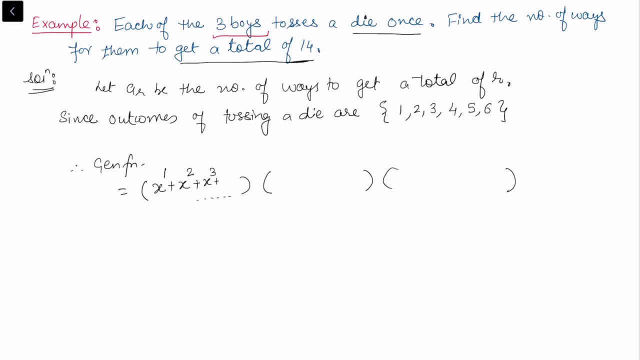 And we know they cannot be infinite. So this particular, when we say x raised to power, n is coming, and then infinite, that means that object can repeat as many as Number of time, but here this is like the size of the occurrence. So it will have to be x to the power 5, and then we will have one more term plus x to the power 6, and similarly the case for the other boy, and similarly is the case for the third boy. 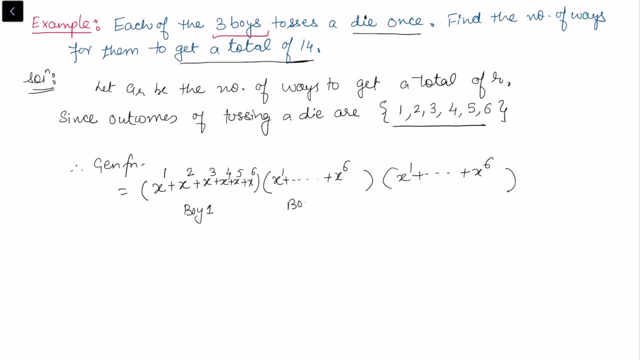 So this we can say for boy 1, for boy 2, and this one is for boy 3, knife edges club. this this will become x to the power 1 square, And then you take cube and so on, plus x to the power 6 whole, raised to power 3, and now we can take x, cube, common, and inside we will have 1 plus x, plus up till so on, plus x to the power 5, whole cube, and so this becomes like a finite geometric progression. 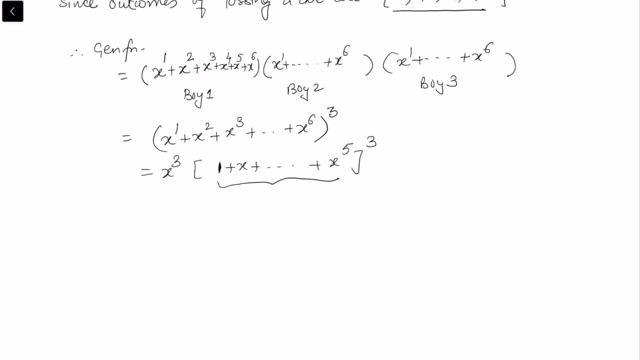 So and the common ratio is x, the first term is 1, so we can apply this formula x cube into 1 minus x to the power 6 over 1 minus x whole cube. Now this is same as x cube and now, if you just open this term, what we can see is we have 1 minus x to the power 6 whole cube and then we can have 1 over 1 minus x whole cube. 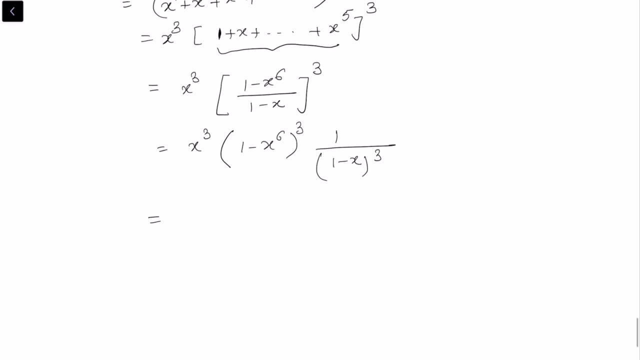 So I've just separated numerator and denominator and if I just open this term, 1 minus x raised to power 6, whole cube. So we can simply open it by the formula a minus b whole cube. So this becomes 1 minus 3 times x to the power, 6 plus 3 times x squared. 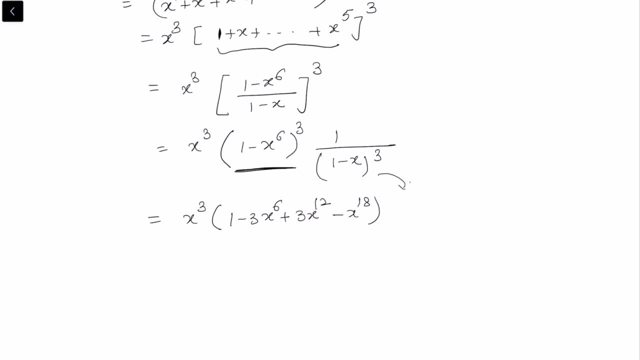 Minus x to the power 18 and this term will become summation i varying from 0 to infinity: i plus 2. choose 2 x to the power i. So this is simply using the binomial theorem. Now again, if I just multiply this x cube inside, so we will have here x cube minus 3 times x to the power 9 exponent. get added plus 3 times x to the power 15, minus x to the power 21.. 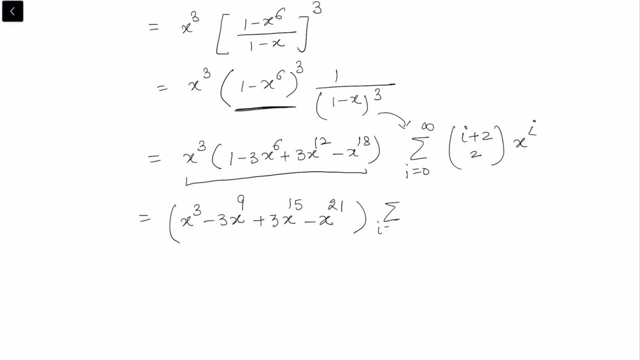 21. And then we take summation i varying from 0 to infinity, i plus 2. choose 2 x to the power i. Now we want to find the coefficient when r is equal to 14.. So we can say: 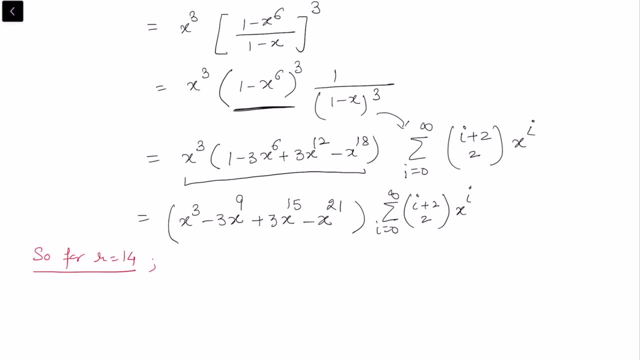 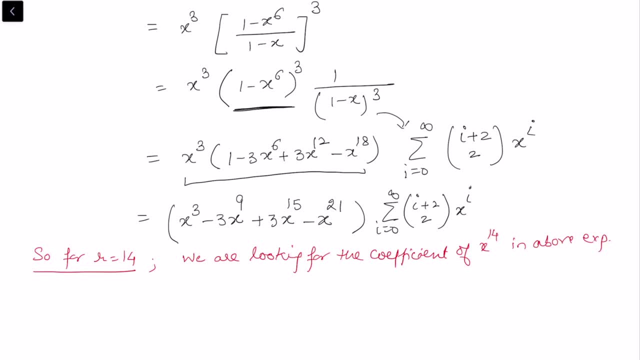 14., 14., 14., 14., 14. 14.. In above expression. in above expression. So we don't want to open the whole terms. and then look: what is the coefficient of x to the power 14? rather, I will use again the previous technique. 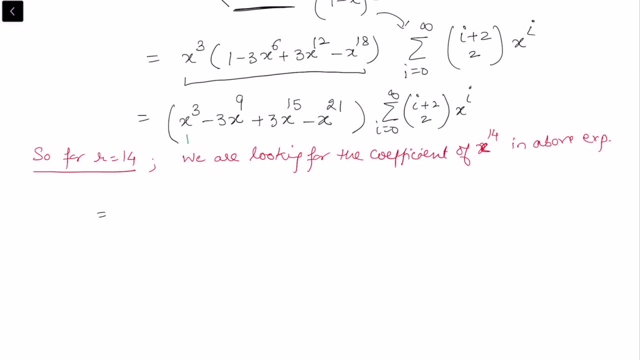 So we will simply look at the expression. So this x cube, when multiplied by this expression, So there is these are the like product of two finite expansion. So on one side we have infinite expansion, but this one is finite, which I highlighted with the green color. and here, when this first term x cube is multiplied by something, 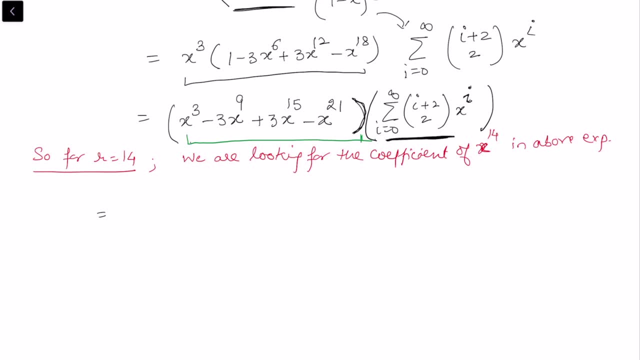 x to the power i, because here I will vary from 0 to infinity. So x cube multiplied by this term will give me the coefficient of x to the power 14 only when I will select x to the power 11 from the second expression, because then x to the power 11 from the second bracket and x to the power 3 from the first one will make a coefficient of x, will make the x to the power 14.. 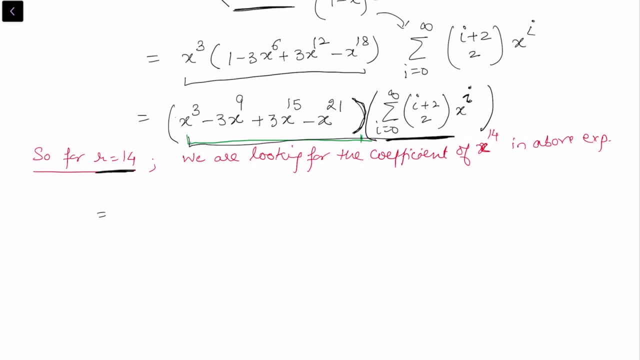 So this means- and we also notice that here the coefficient is 1.. x cubes coefficient is 1.. So this means all the contribution of the coefficient will come from here only, and in this case the i should be 11 plus 2. choose 2.. 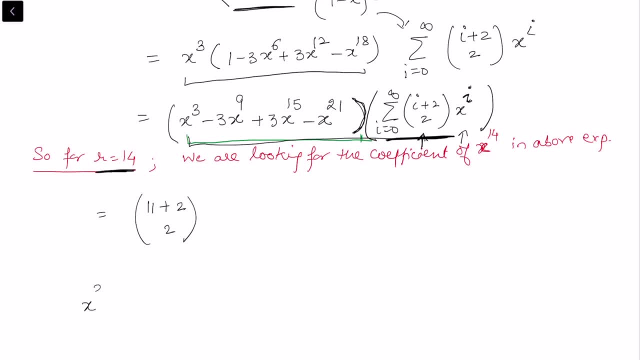 So I am looking here, I can write this first term like x cube, So this is the first term multiplied here. So if I just open the summation, this will be 2, choose 2. when i is equal to 1, x to the power, 0 plus. then if i is equal to 1.. 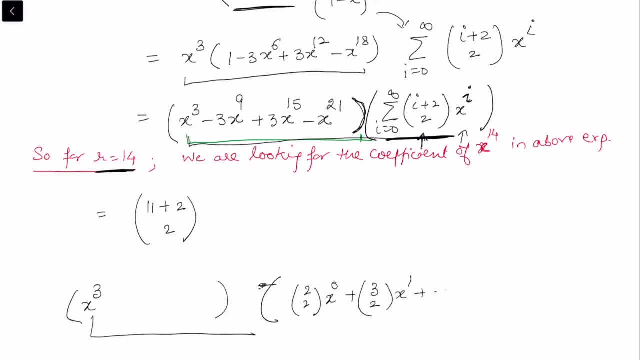 This will be 3- choose 2, x to the power 1, and we continue, and then there will be a term when i is equal to 11 plus 2- choose 2 and x to the power 11, and we continue doing like this one. 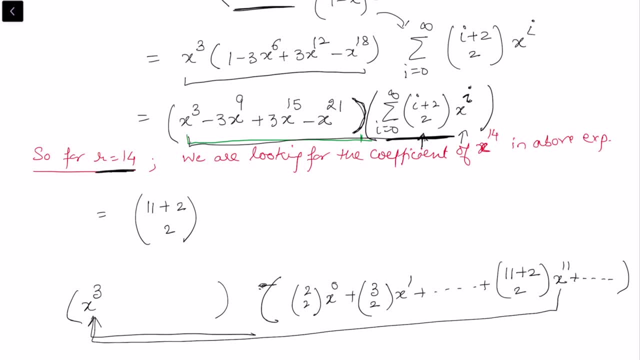 Now this x to the power 11, when multiplied by this x cube, will make a total of x to the power 14. and this is what we are looking and corresponding to this multiplication we see here, the coefficient is 1.. So this 1 is multiplied by x cube. 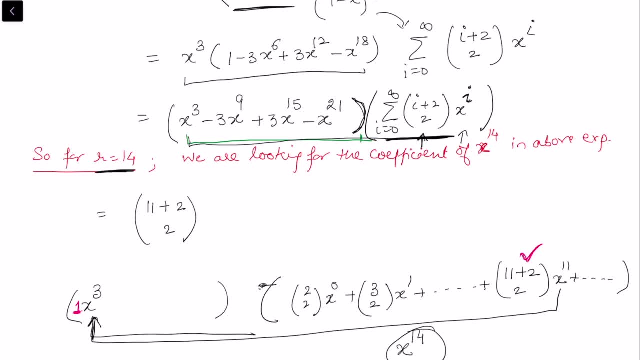 So this is the first term multiplied by this term: 11 plus 2, choose 2.. So that is why I have written for the first term- 11 plus 2, choose 2- and similarly we look for the product of the other case.